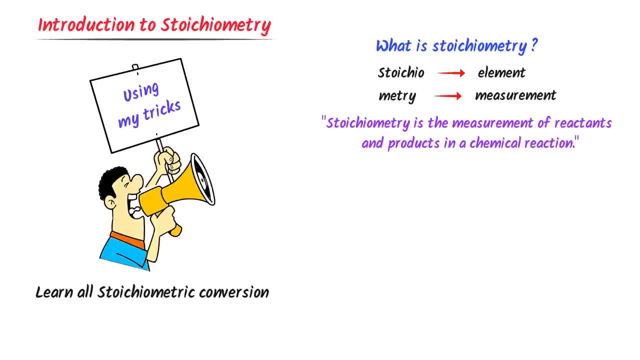 calculation of products and reactants and a chemical reaction. For example, consider this general chemical reaction. With the help of strychometry we can find the number of moles of reactants and the number of moles of products. So remember that strychometry is the calculation. 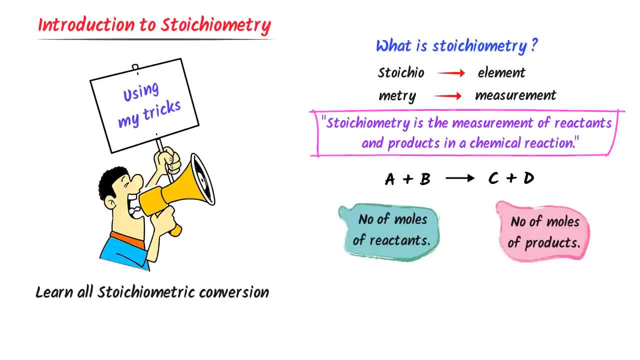 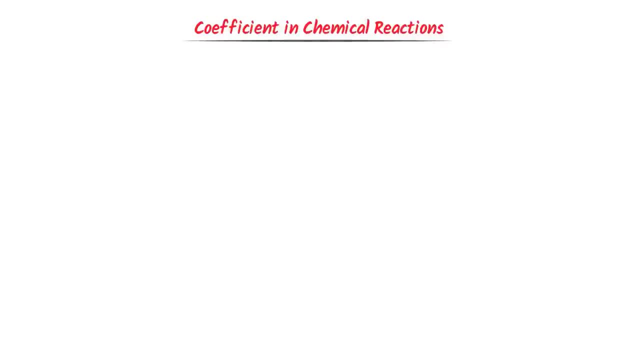 of products and reactants and a chemical reaction. Now let me teach you the important concept of coefficients and a chemical reaction, which a lot of students are not understanding. For example, consider this chemical reaction. Now I will balance this chemical reaction. There are two hydrogen atoms and the reactants. 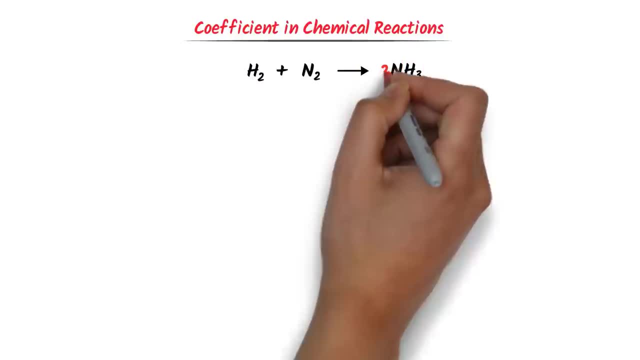 Well, there are three hydrogen atoms and the products I place: two with products and three with the reactants. Now, 3 into 2 is equal to 6 atoms. 2 into 3 is equal to 6 atoms. There are: 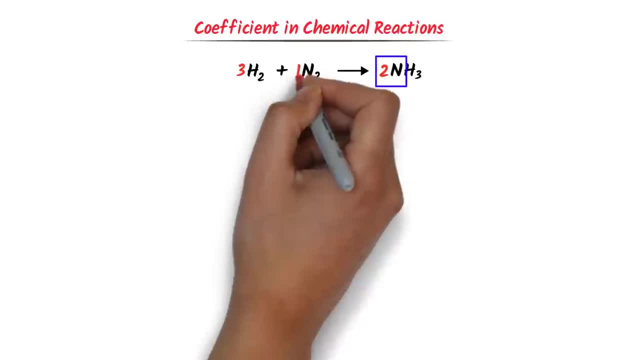 two nitrogen atoms and there are also two nitrogen atoms. Now I will balance this chemical reaction. So this is complete, balanced chemical reaction. Now, this three with hydrogen gas is known as coefficient of hydrogen gas. Secondly, this one with nitrogen gas is known as coefficient of 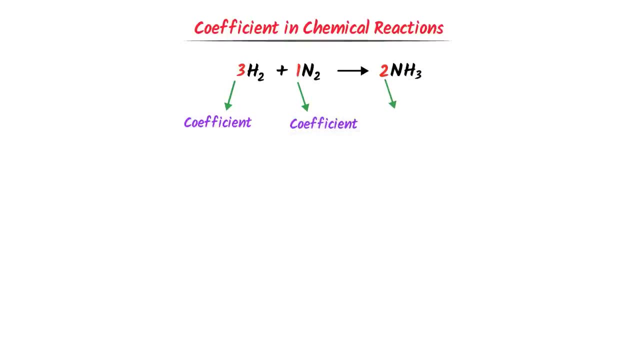 nitrogen gas, While this two with NH3 is known as coefficient of NH3.. Here I will teach you three different stories of coefficients. Firstly, the coefficients represents the amount of substances. For example, this three coefficient of hydrogen gas shows three moles of hydrogen gas. 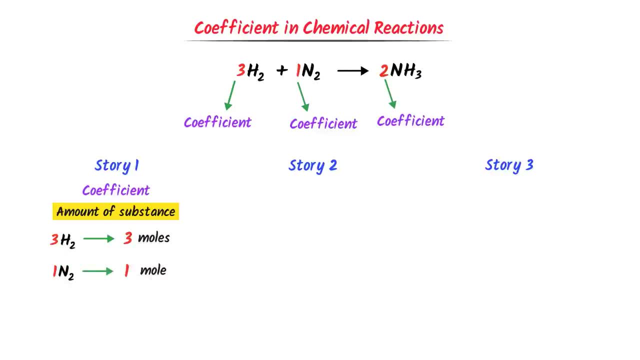 One coefficient of nitrogen gas represents one mole of nitrogen gas And two coefficient of NH3 represents two moles of NH3.. Secondly, coefficients represent a ratio of reactants to products. For example, I write hydrogen gas ratio to nitrogen gas to NH3. 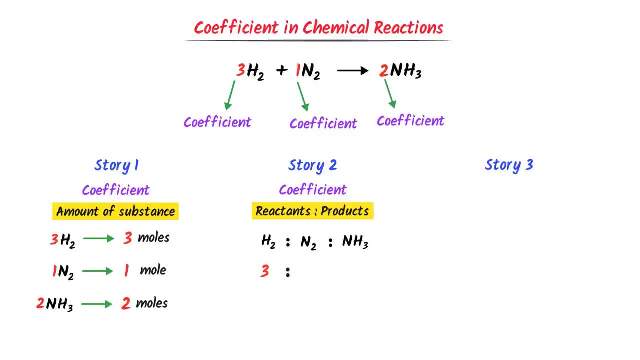 Now that the coefficient of hydrogen gas is three, that of nitrogen gas is one and that of NH3 is two. Hence, this is the ratio of reactants to products. Thirdly, coefficients represents number of molecules. Let I write three hydrogen gas, one nitrogen gas, two NH3.. Now this three coefficient of hydrogen gas. 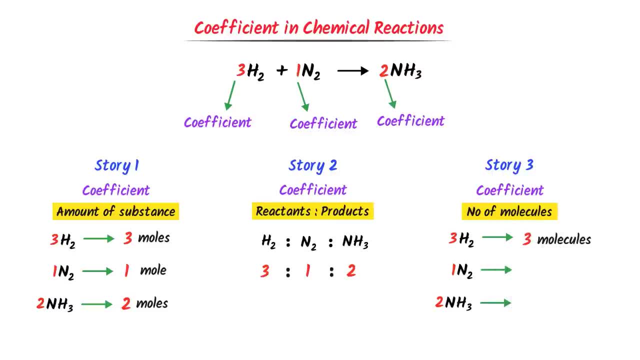 represents three molecules of hydrogen gas. For example, I write oneför dope, two NOs, two null. Thus I write: one1 estou and the ratio of reactants to products represents the SO. Thus I write: the ratio of reactants to products is one容. 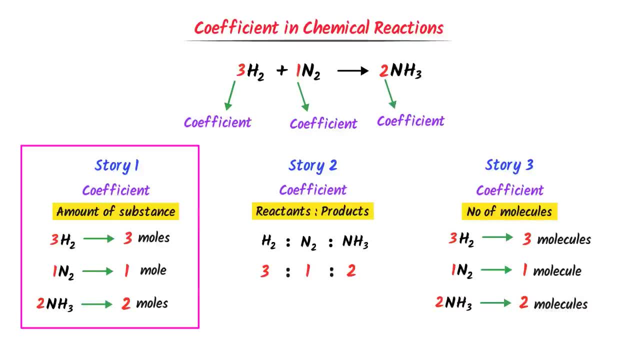 Just remember that story one tells that the coefficient represents the number of moles. Story two tells that the coefficient represents the ratio of reactants to the products. Just remember that. story 3 tells that the coefficient represents the number of moles. the coefficient represent the number of molecules. 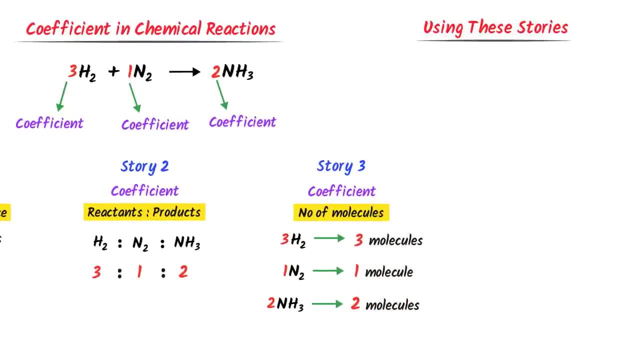 Now, how can we use these stories to calculate the amount of reactants and products? Well, consider this question: How can you form 6 molecules of NH3?? The answer is simple. According to the second story, the ratio of hydrogen to nitrogen to NH3 is 3 to 1,, 1 to 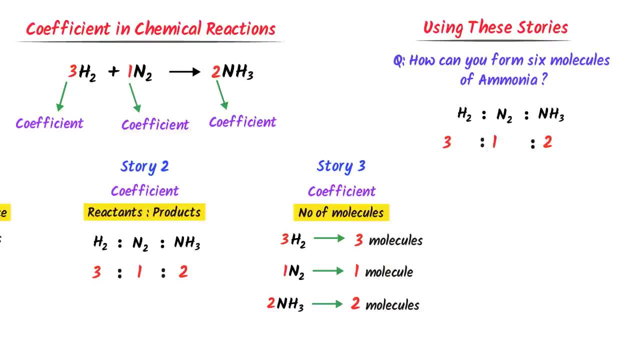 2. We need 6 molecules of NH3.. I just multiply 2N to 3.. I also multiply the ratio of N2 by 3 and that of H2 by 3.. Now, 2N to 3 is equal to 6, 1N to 3 is equal to 3, 3N to 3 is equal to 9.. 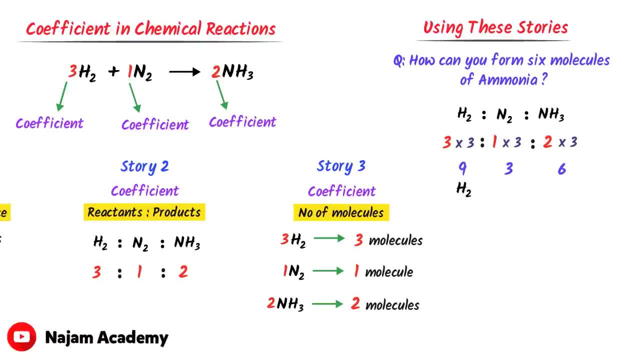 This reveals that we need 9 molecules of hydrogen gas to react with 3 molecules of nitrogen gas in order to form 6 molecules of NH3.. Let me repeat this question: We need 9 molecules of hydrogen gas to react with 3 molecules of nitrogen gas in order. 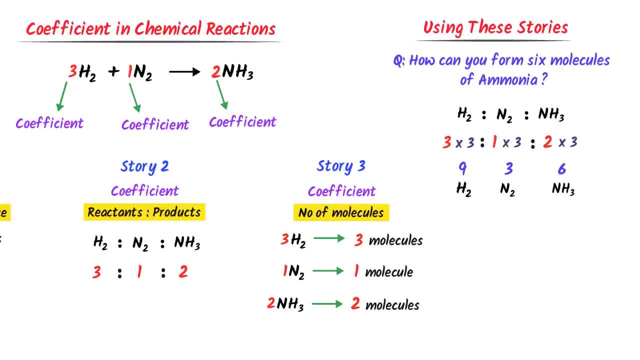 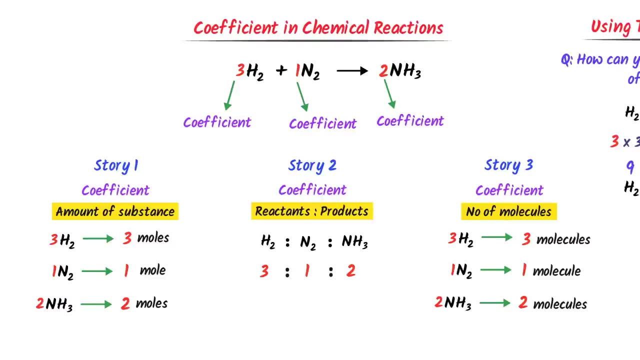 to form 6 molecules of NH3.. To conclude this whole concept, any coefficient in a reaction shows either number of moles, a ratio or number of molecules. and snorted down all these important concepts, Now let me teach you the different conversions of stoichiometry. 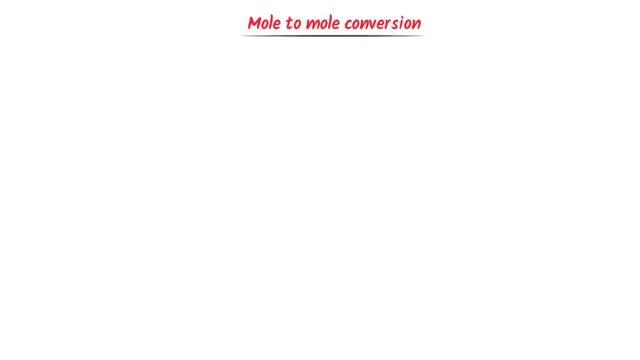 Consider this problem: How many moles of nitrogen gas is needed to react with 13.5 moles of hydrogen to form NH3?? Well, I write the balanced chemical reaction. We know that hydrogen gas plus nitrogen gas react together to form NH3. 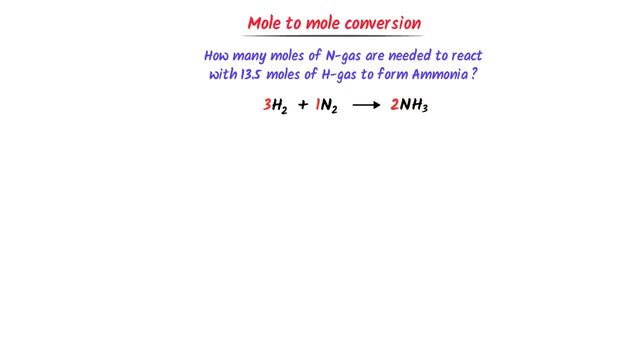 I put here 3,, 1 and 2.. This is the complete balanced chemical reaction. Now, according to the given statement, 13.5 moles of hydrogen gas is given. We need to find the number of moles of nitrogen gas. 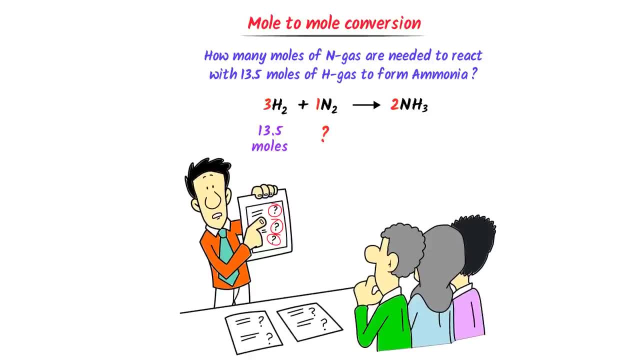 Although there are several ways to calculate it. but I will teach you my way to calculate such type of questions. Firstly, I write ratio of hydrogen to the ratio of nitrogen gas. We know that it is 3 to 1.. Now listen carefully. 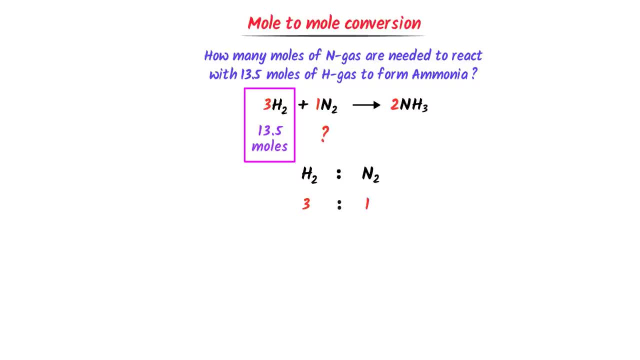 We are already given the number of moles of nitrogen gas. We know that it is 3 to 1.. We are already given the number of moles of hydrogen. I will write this: 13.5 moles below the hydrogen gas. 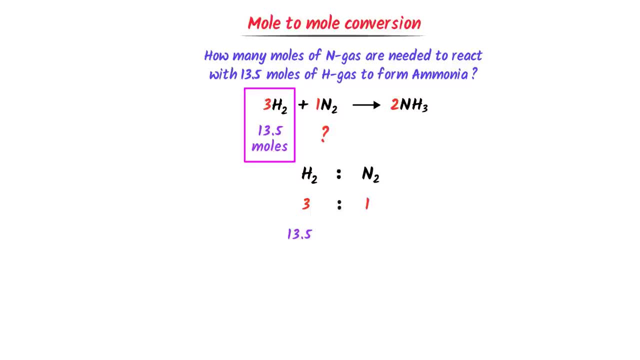 Let me repeat it: We are already given the number of moles of hydrogen gas. I will write this 13.5 moles below this hydrogen gas Here. if 3 moles of hydrogen gas react with 1 mole, then 13.5 moles of hydrogen gas react. 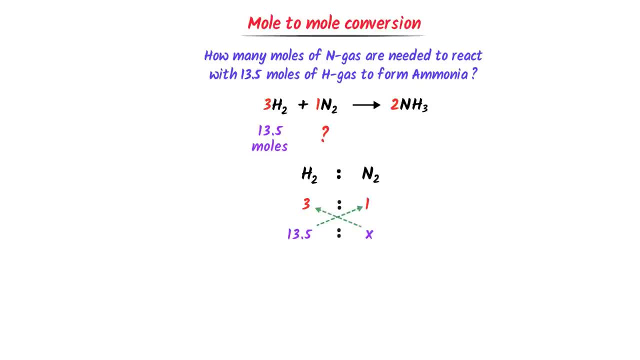 with x moles. Now I will just cross: multiply 3 x x is equal to 1 x 13.5.. I divide both sides by 3.. After calculation I get x is equal to 4.5 moles. 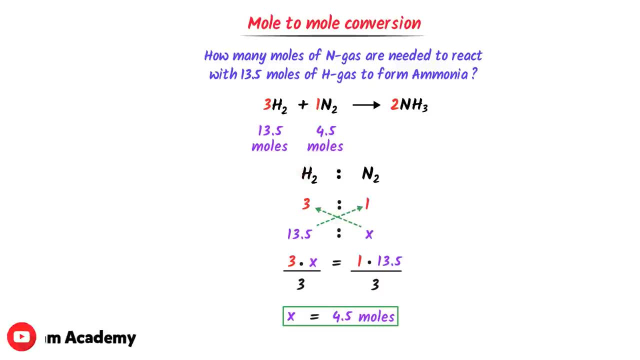 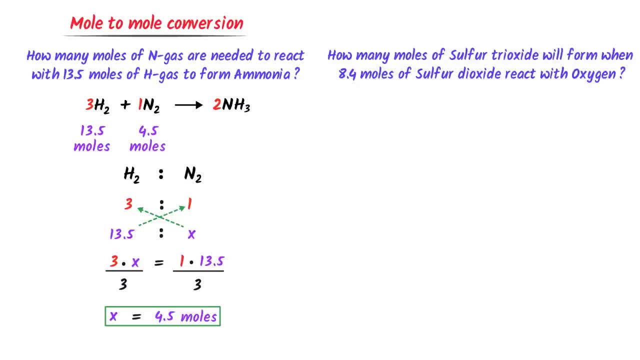 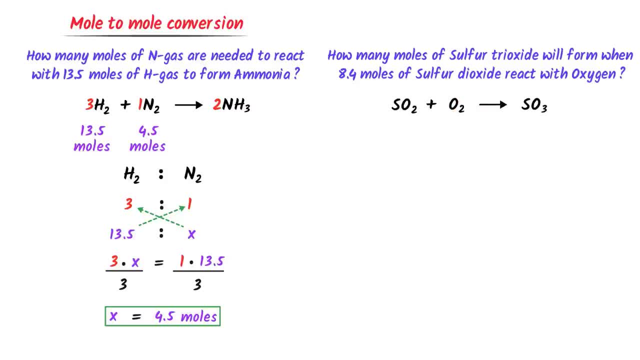 Here comes the big problem. Fourth problem: This is the cavasary reaction, which requires Radix, dop, euh and avonsела. good result in 4.5 moles alpha and in the finalはいうこと I have expressed again. 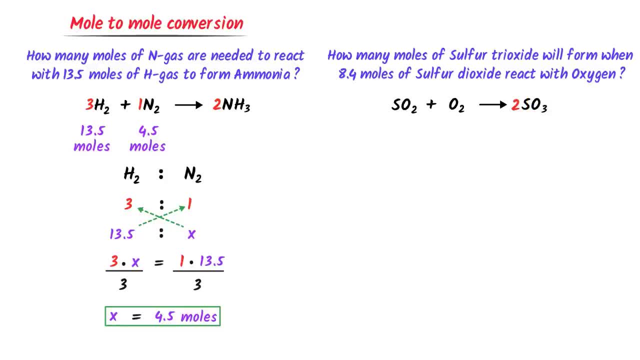 this is a attribüssel. I have return the value to zl, I place here 2, and the product. there are 2 sulfur atoms and the reactant, I place here 2.. Hence, this is the complete, balanced chemical equation. According to the given statement, 8.4 moles of sulfur dioxide will react with oxygen to. 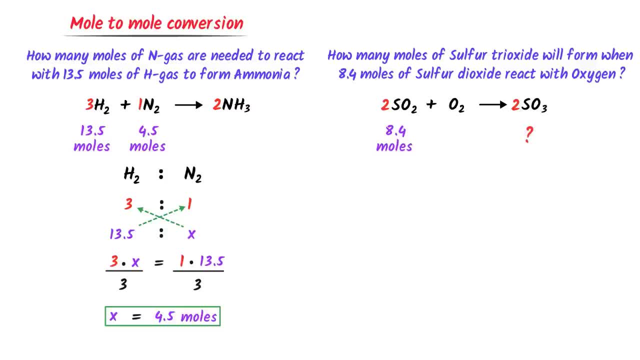 form x: moles of sulfur trioxide. Now I will use my personal way to calculate the number of moles of sulfur trioxide. I establish ratio between sulfur dioxide and sulfur trioxide. We can see that it is 2 ratio to 2.. 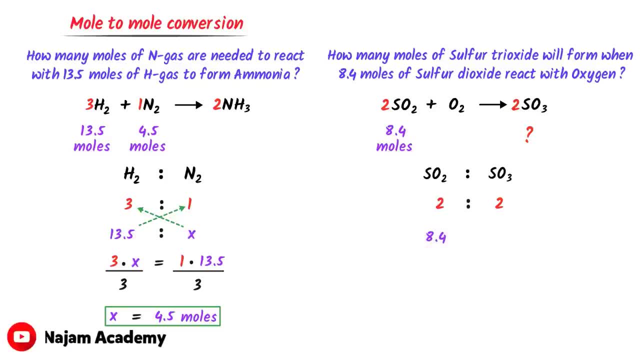 The number of moles of sulfur dioxide is 8.4 moles. We need to calculate the number of moles of sulfur trioxide. Let it is x Now I cross. multiply them: 2n to x is equal to 2n to 8.4.. 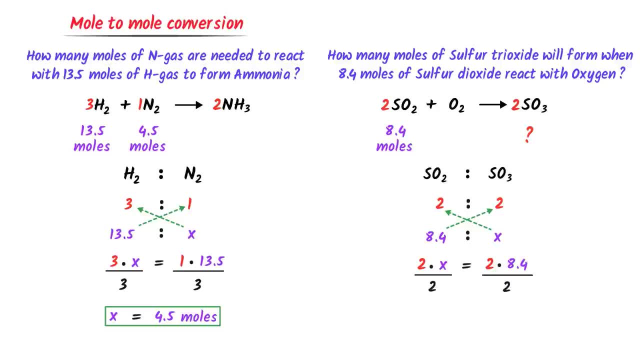 I divide both sides by 2. After calculation, I get 8.4 moles. Thus, 8.4 moles of sulfur dioxide will react with excess of oxygen to form 8.4 moles of sulfur trioxide. Hence noted down this important problem. 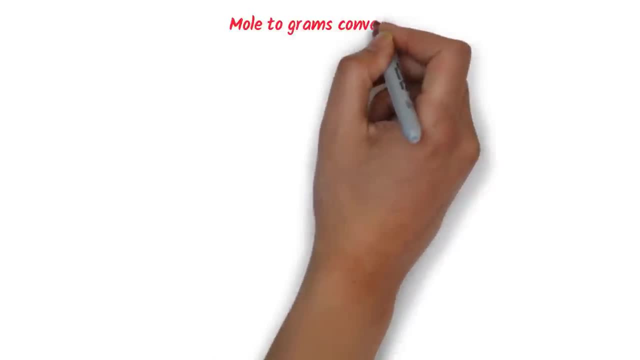 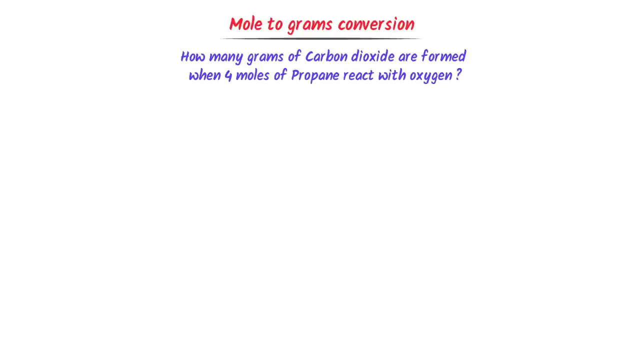 The second type of stoichiometric conversion is mole to gram conversion, For example. consider this problem. Firstly, I write the complete balanced chemical reaction. According to the given statement, propane C3H8 react with oxygen to form carbon dioxide plus water. 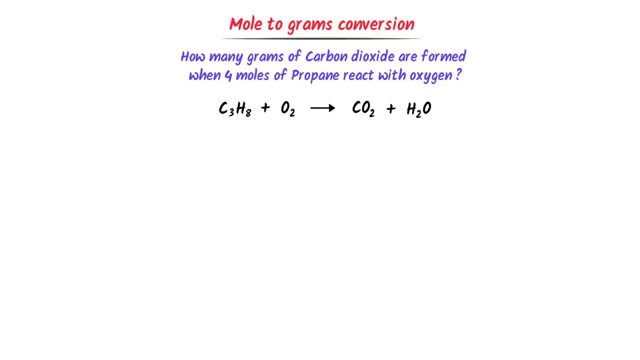 It is a simple combustion reaction. Now there are 3 carbons in the reactants and 1 carbon in the products I place here 3.. There are 8 hydrogen in the reactants and 2 hydrogen in the products I place here 4.. 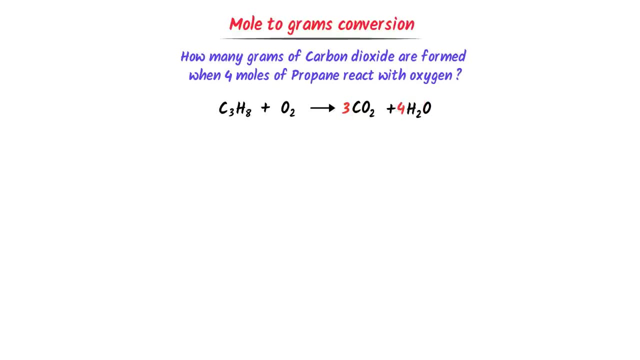 2n to 4 is equal to 8 hydrogen atoms. Now 2n to 3 is equal to 6 oxygen atoms. plus 4 oxygen atoms is equal to 10 oxygen atoms. I write here 5.. Hence this is the complete, balanced chemical equation. 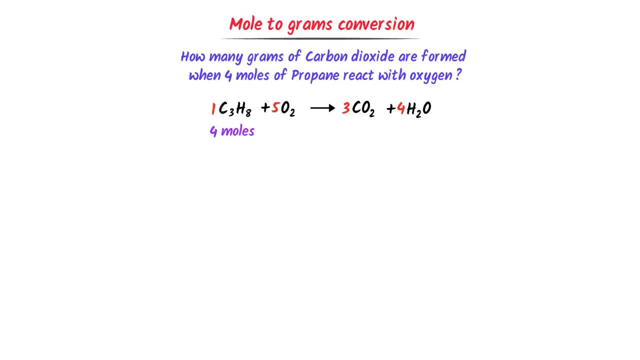 Now, 4 moles of propane will react with oxygen to form x grams of carbon dioxide. Although there are several ways to calculate it, but I will use my personal way, I solve this type of problem in two steps. In the first step, I find the number of moles of unknown species like carbon dioxide. 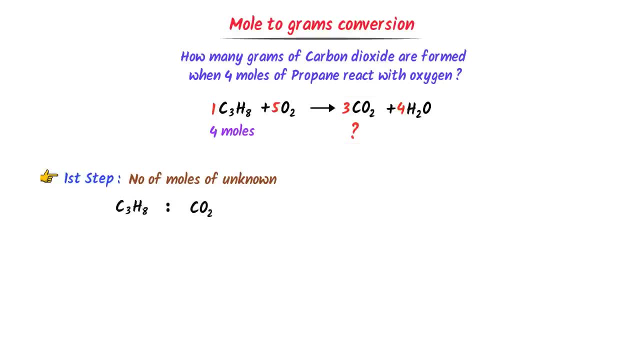 I establish relationship of ratio between propane and carbon dioxide. We can see that it is 1 to 3.. 4 moles of propane is given and the moles of carbon dioxide is unknown. I have to cross multiply them. 1n to x is equal to 4n to 3.. I have to cross multiply them. 1n to x is equal to 4n to 3.. I have to cross multiply them. 1n to x is equal to 4n to 3.. I have to cross multiply them. 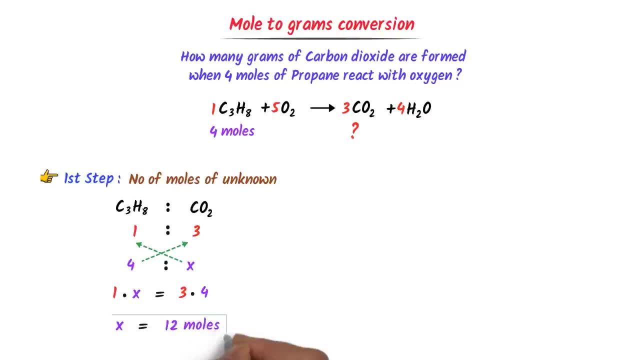 After calculation I get: x is equal to 12 moles of carbon dioxide. Hence, 4 moles of propane will react with oxygen to form 12 moles of carbon dioxide. Let me repeat it: 4 moles of propane will react with oxygen to form 12 moles of carbon dioxide. 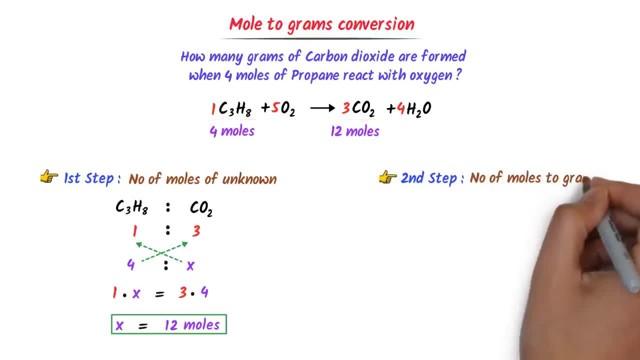 In the second step I just convert the number of moles to grams. The number of moles of carbon dioxide is 12 moles, 12 moles which we calculated. Now the molar mass of carbon dioxide is 44 gram. 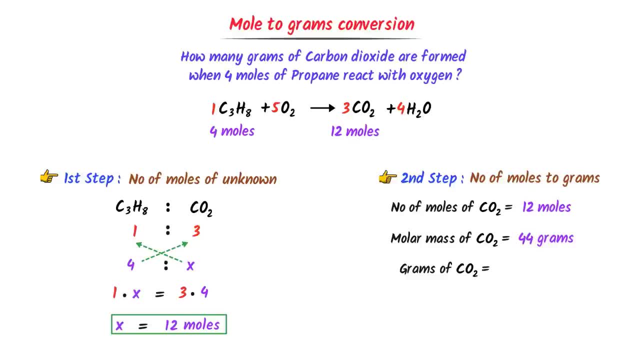 To convert the number of moles of carbon dioxide to grams, I use this formula: Number of moles into molar mass. We know that the number of moles of carbon dioxide is 12 moles into the molar mass of carbon dioxide is 44 gram. 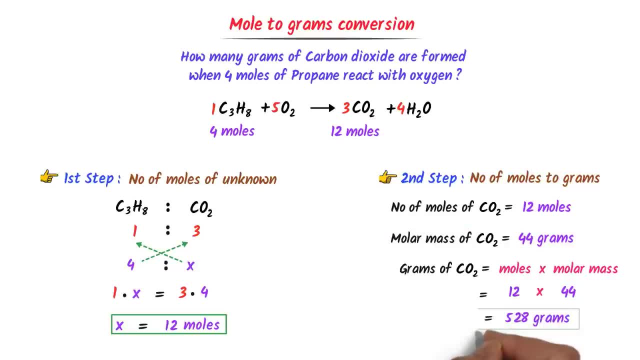 After calculation I get 528 grams of carbon dioxide. Therefore we say that 4 moles of propane will react with oxygen to form 528 grams of carbon dioxide. In such type of problems, I convert given number of moles to moles of unknown species. 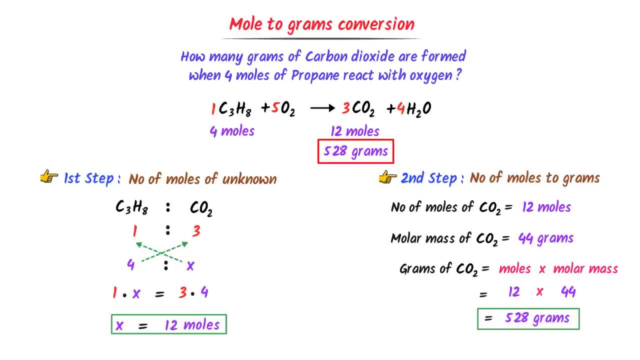 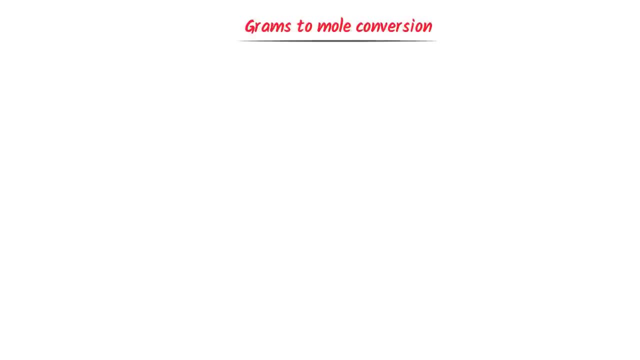 Then I convert number of moles to grams. Hence noted down this important conversion. The third type of stoichiometric conversion is grams to mole conversion. Consider this problem: How many moles of hydrogen are necessary to react with 6 grams of nitrogen to produce? 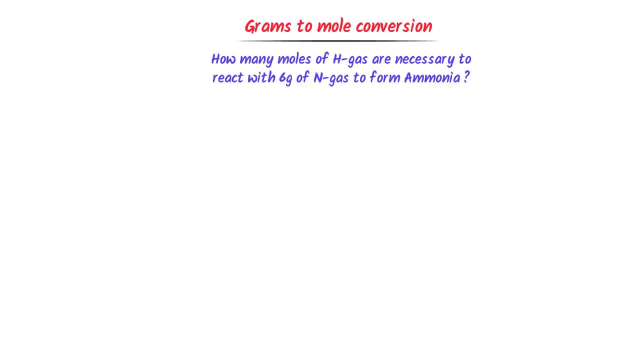 NH3?? Well, as usual, I write balanced chemical reaction. Hydrogen gas plus nitrogen gas will react together to form NH3. I put here 3, 1 and 2.. This is the complete balanced chemical equation. I have completed the equation. 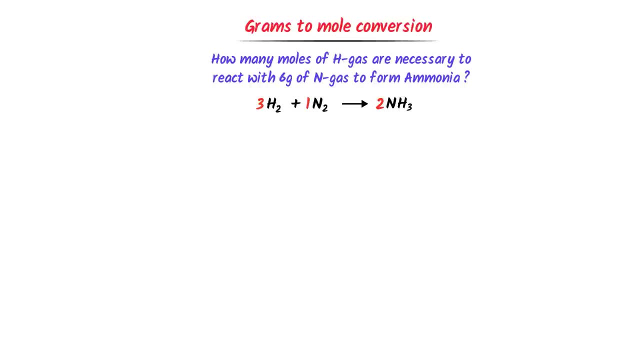 To solve these type of stoichiometric problems, I follow two steps. In the first step, I convert the given mass to mole of the known species. For example, 6 gm of nitrogen gas is given and we have to find x moles of hydrogen gas. 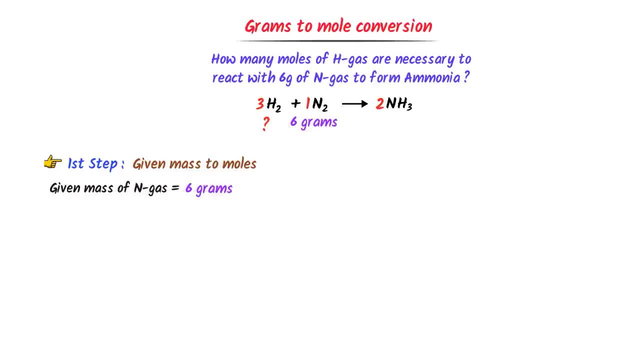 We know that the given mass of nitrogen gas is 6 gm and the molar mass of nitrogen gas is 28 gm. Now I will use this formula to find the number of moles of nitrogen gas given mass upon molar mass. 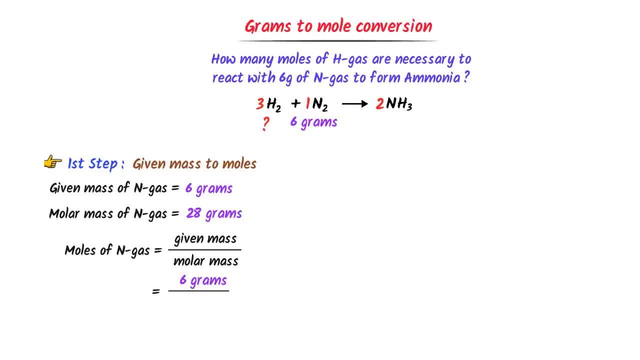 The given mass of nitrogen is 6 gm and the molar mass of nitrogen gas is 28 gm. After calculation I get 0.23 moles of nitrogen gas, Hence 6 gm, or 0.23 moles of nitrogen gas. react with x mole. 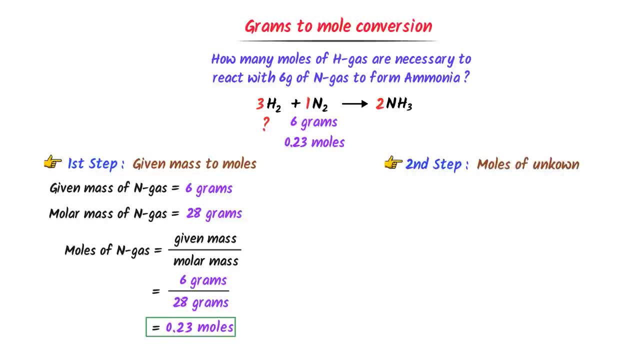 In the second step I will find the number of moles of unknown species Like hydrogen gas. I establish relationship of ratio between hydrogen gas and nitrogen gas. It is 3 to 1. We know that 0.23 moles of nitrogen gas react with x moles of hydrogen gas. 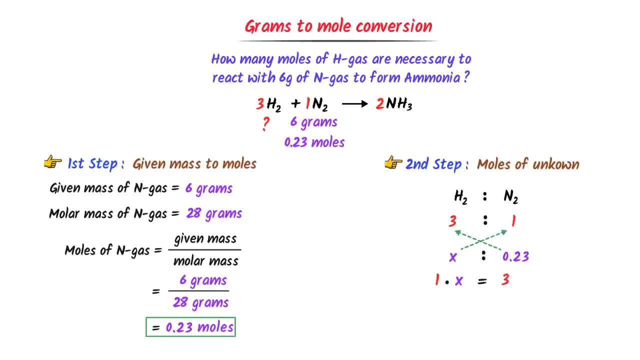 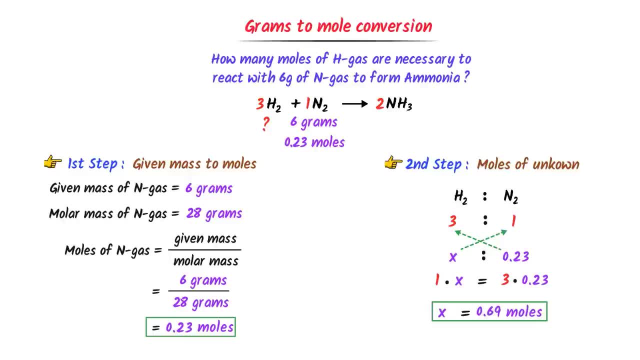 So x is equal to 0.23 moles. Therefore 6 gm of nitrogen gas will react with 0.69 moles of hydrogen gas to produce NH3.. In such type of problems I convert given mass to number of moles. 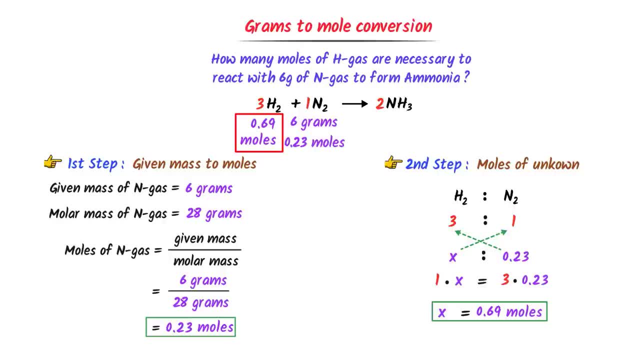 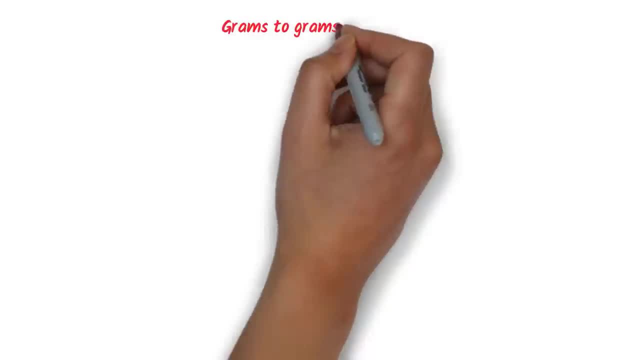 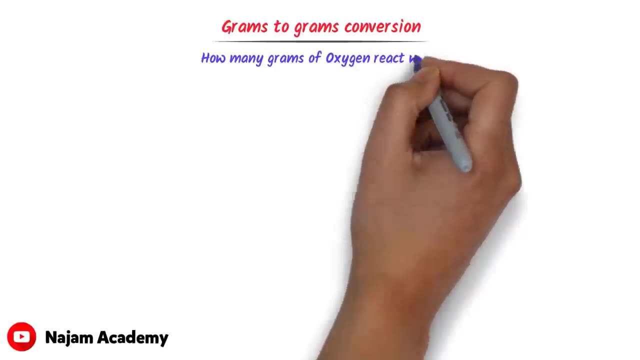 Then I convert number of moles to number of moles of unknown species. Hence, noted down this important conversion. Lastly, let me teach you grams to grams conversion. For example, consider this problem: How many grams of oxygen react with 10 grams of hydrogen gas to form H2O? 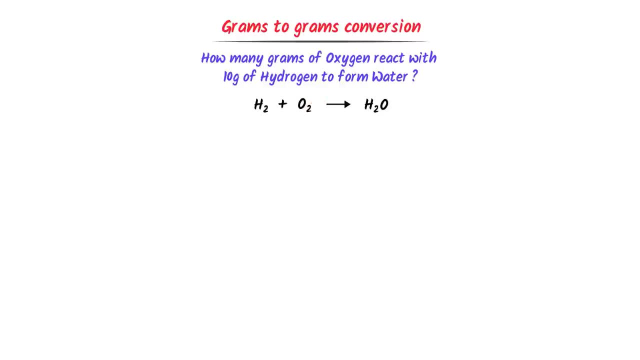 Well, as usual, I write the complete balanced chemical equation. Hydrogen gas plus oxygen gas react together to form water. I write 2,, 1 and 2.. Now it is a complete balanced chemical reaction. Here the mass of hydrogen gas is given, which is 10 grams. 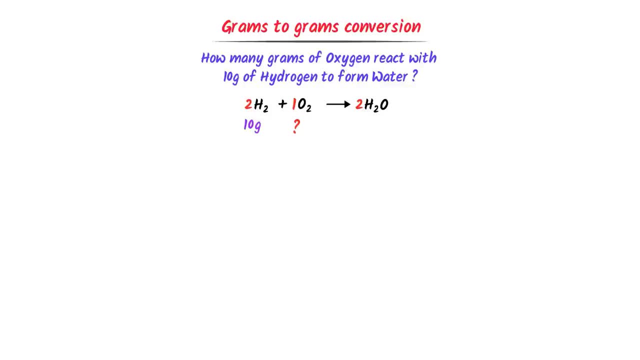 I need to find the mass of oxygen gas. Also, I need to find the number of moles of hydrogen gas and oxygen gas. Firstly, I find the molar mass of hydrogen gas, oxygen gas and H2O. The molar mass of hydrogen gas is 2 gram, that of oxygen gas is 32 gram and that of 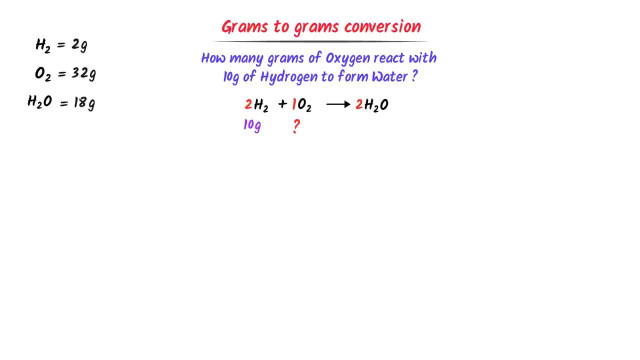 water is 18 gram. Now I will follow these three steps. In the first step, I will find number of moles of non-species like hydrogen gas. I use this formula: Number of moles of hydrogen gas is equal to given mass upon molar mass. 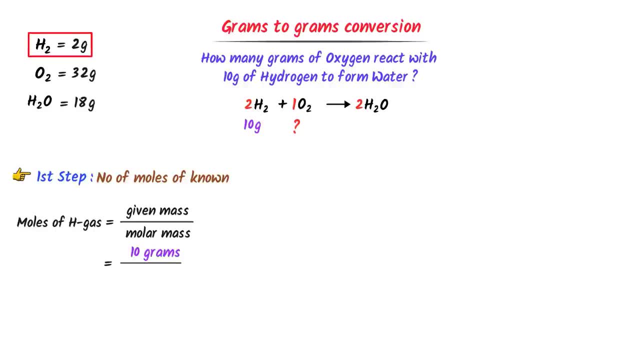 The given mass of hydrogen gas is 10 gram and its molar mass is 2 gram. After calculation I get 5 moles of hydrogen gas. Thus 10 gram are 5 moles of hydrogen gas. react: The given mass of hydrogen gas is equal to given mass upon molar mass. 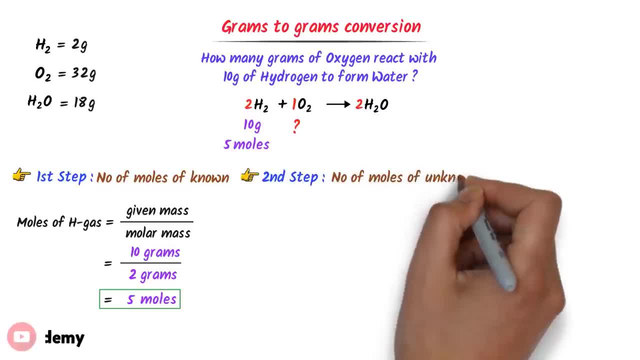 The given mass of hydrogen gas is equal to given mass upon molar mass. In the second step, I find the number of moles of unknown species like oxygen gas. To do so, I establish relationship of ratio between hydrogen gas and oxygen gas.